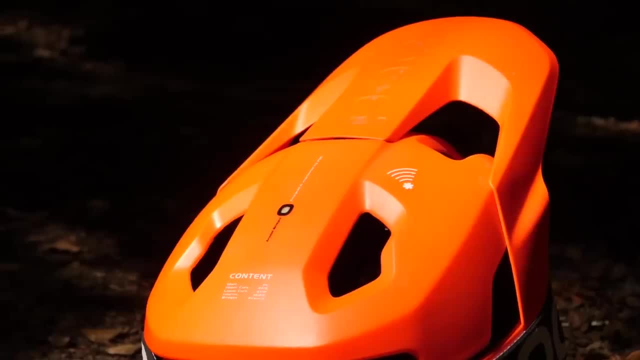 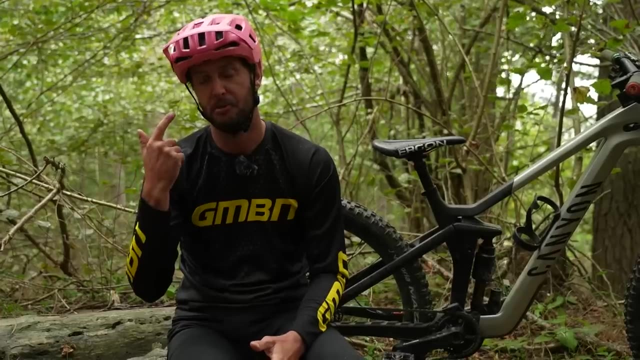 and full-on downhill versions being a little more lighter weight and more vented, The bigger ones definitely a bit more heavy-duty. if you're really putting the laps in. If you want to protect the eyeballs, glasses and goggles are an absolute must. if you're not, 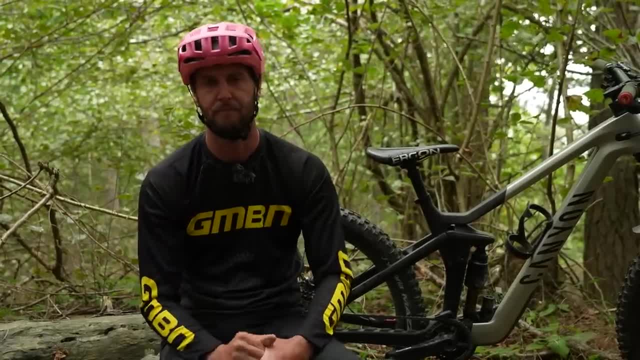 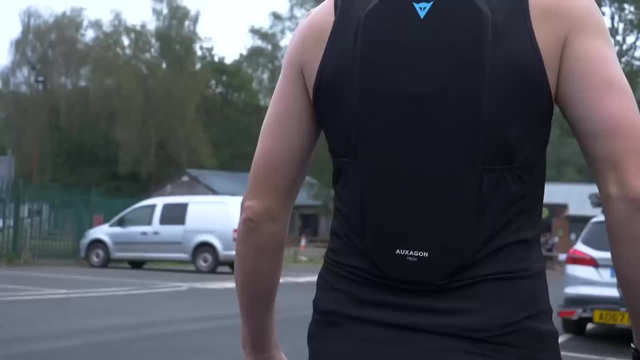 too fussed. Also, stop teary-eyed, stop you getting emotional on the way down. For safety, you might want to think about wearing a body armor. so certainly a chest protector maybe, but definitely a back protector. if that is your thing, It can help with confidence. 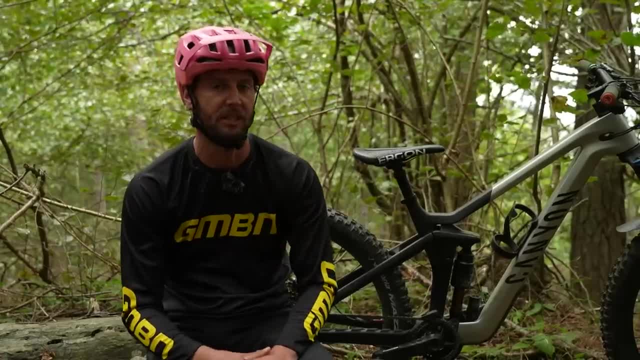 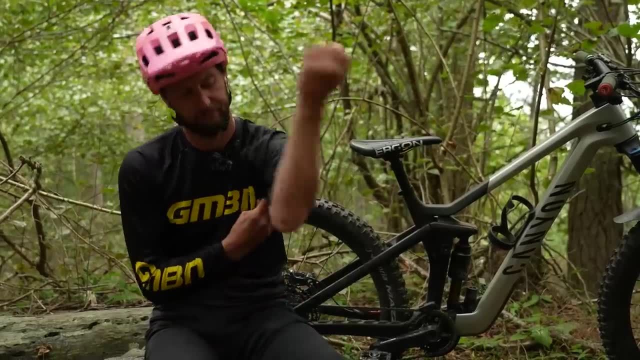 There are certain versions of this as well. Check the CE certificate on these, though, to make sure that they are up to scratch. Elbow pads are another one. Nobody wants skinned elbows. Look, what's that all about? I could have avoided that if I had elbow pads on. 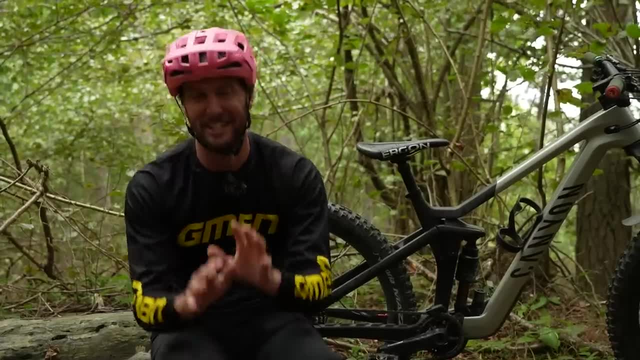 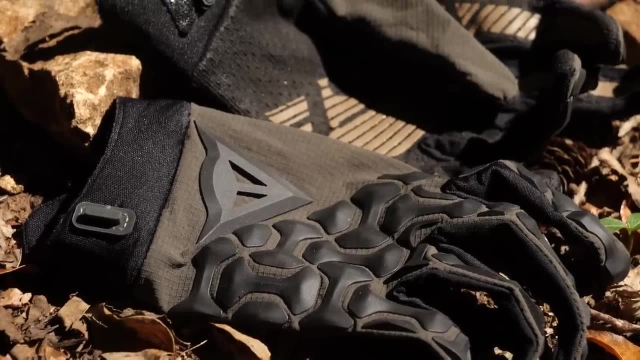 Gloves, of course, as well. Now call me a hypocrite, because I don't wear gloves very often. I know you're all going to tell me off for that, but gloves will stop you shredding your hands. Maybe look at different ones of varying levels of protection on the back and on the palms. 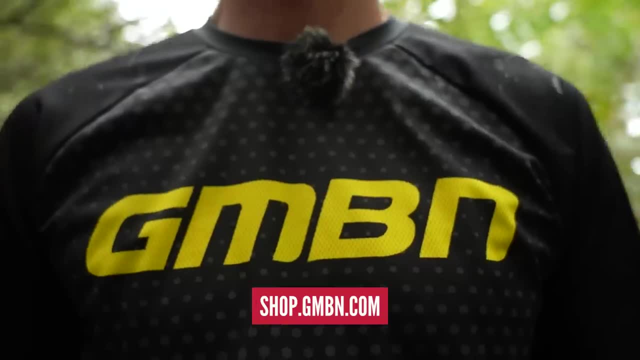 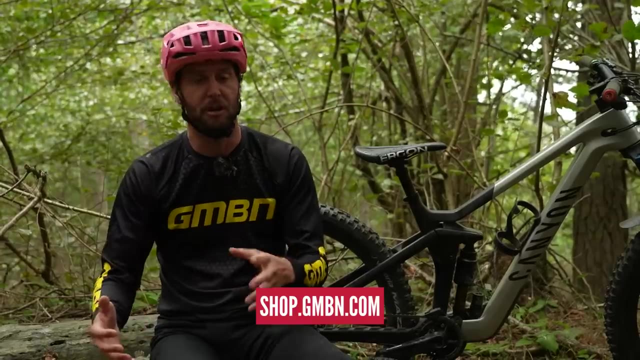 as well. When it comes to jerseys. there are downhill jerseys like this GMBN, available in the shop, one that we've got here, Long sleeve again to help protect you. They're made of tough material to stop ripping and shredding as well. The same with pants. downhill trousers. 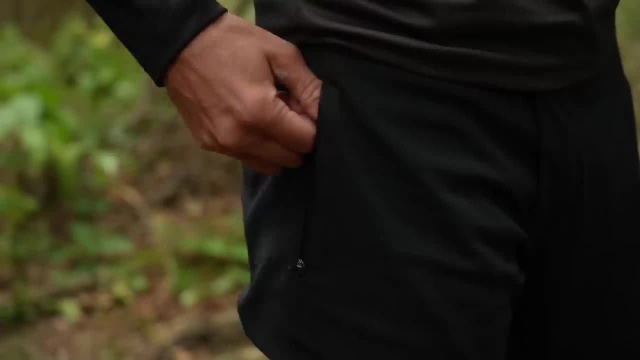 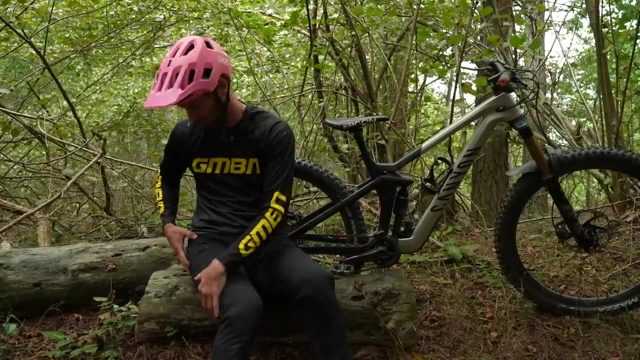 as well. These ones are fairly fitted, these Danes ones, They've got little pockets in those still. Again, they're an abrasion resistant material. You can get padded undershorts to stop your thighs and your hips getting beaten up. Those are always really useful. Then onto. 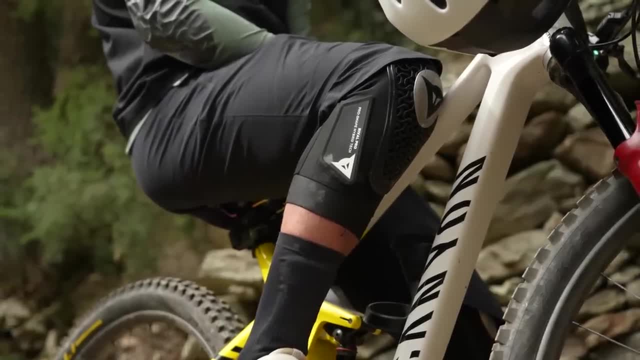 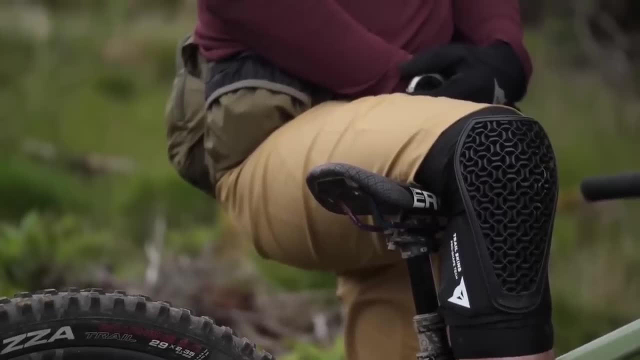 knee pads. Again, like all protection, knee pads come in varying stages of paddedness. I'm not sure that's a word. You can go from a real soft shell knee pad like a sleeve all the way up to a big burly, padded hard shell knee pad as well, which will absorb the biggest craziest. 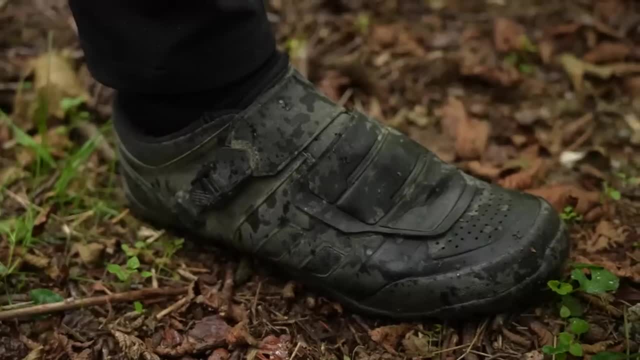 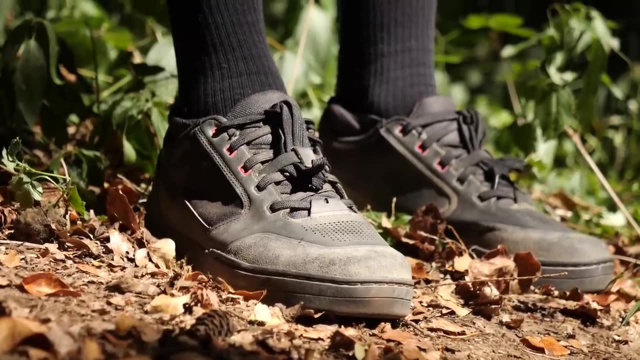 crashes, you can throw at them. Then it's down to your footwear. Don't be fooled by the disco slipper. I wear them now and again, obviously, but a downhill specific style shoe will be much more padded. It will be much tougher material If you bang your foot against rocks. 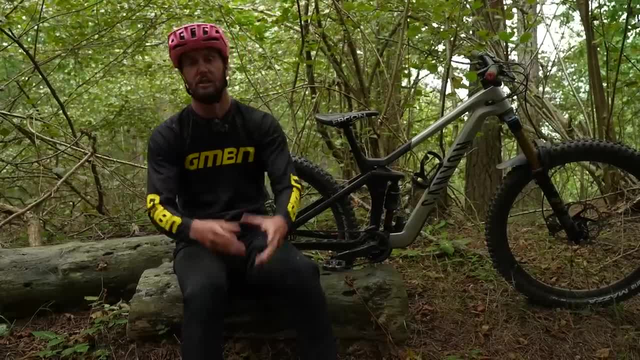 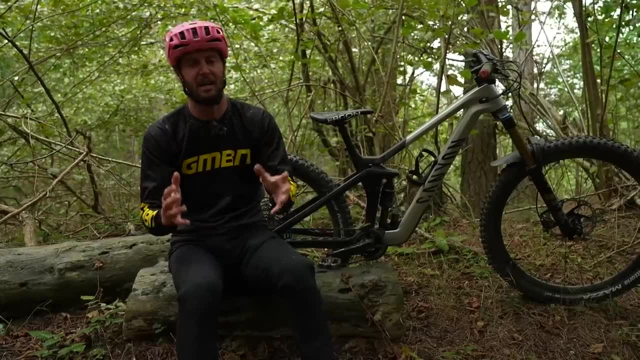 or stub your toes. you're not going to destroy your foot or your shoe. That is a quick run through. Then, when it comes to bike, well, I don't like to tell you what bike to ride. You can ride on any kind of bike, but the more travel, the bigger the brakes, that kind. 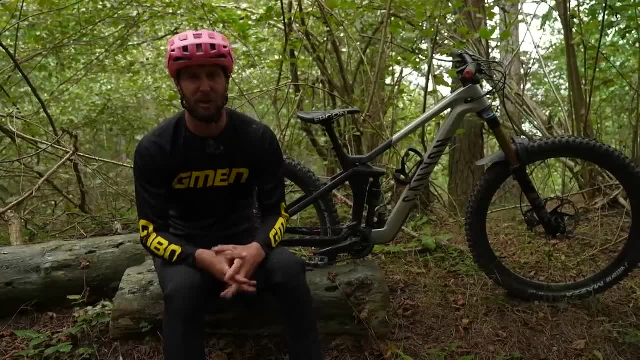 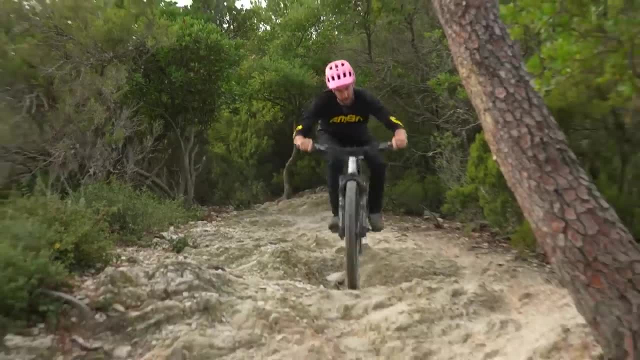 of thing. the weather's coming, the more you're going to enjoy it. Right, that's enough of me talking. Let's go find Loris in the woods to get onto the skills part. Speaker 1. Speaker 2. Speaker 3. Speaker: 4 Speaker, 5 Speaker, 6 Speaker, 7 Speaker, 8 Speaker, 9 Speaker, 10 Speaker, 11 Speaker, 12 Speaker, 13 Speaker, 14 Speaker, 15 Speaker, 16 Speaker, 17 Speaker, 18 Speaker, 19 Speaker 21. 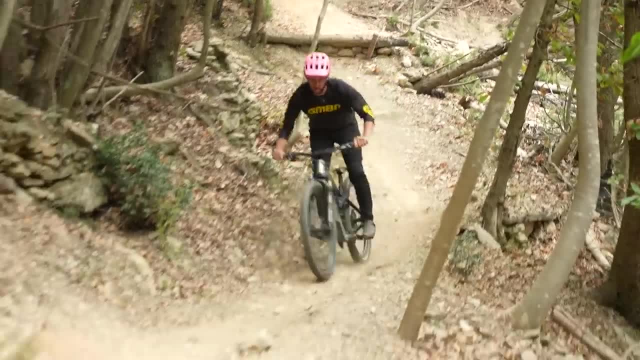 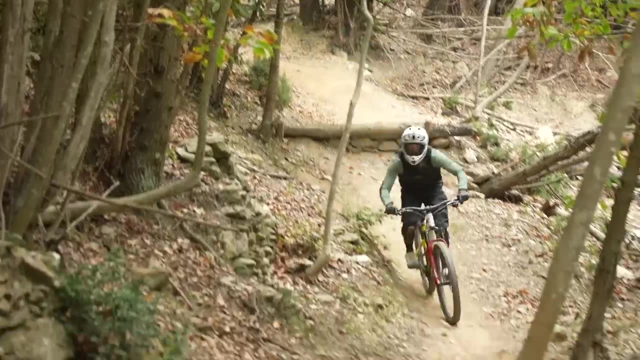 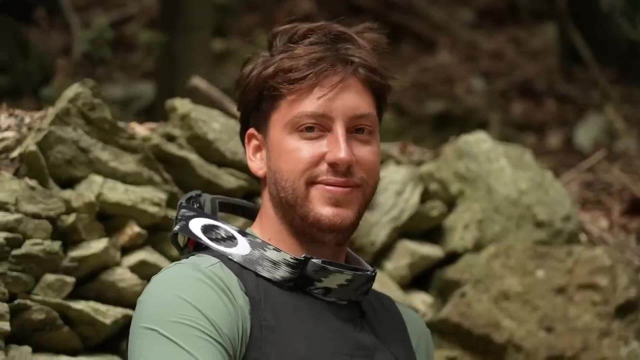 Speaker. 22 Speaker, 23 Speaker. 24 Speaker, 25 Speaker, 26 Speaker, 27 Speaker, 28 Speaker, 29 Speaker, 30 Speaker, 31 Speaker, 31 Speaker, 32 Speaker, 33 Speaker, 34. Look who we've got here: Loris Ravelli. Loris, thank you for joining me, mate. 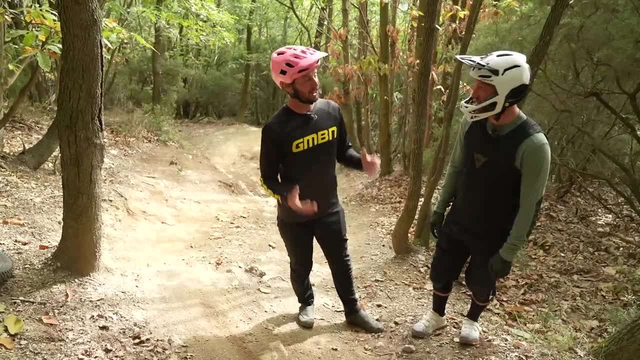 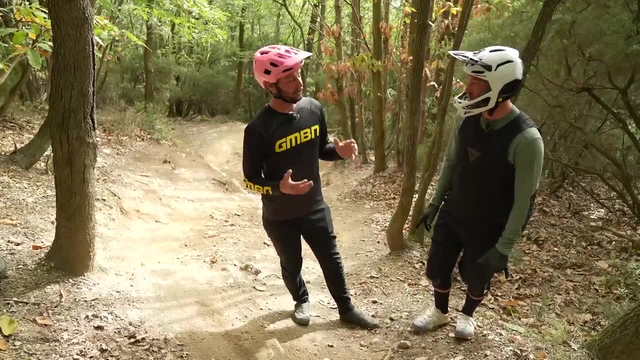 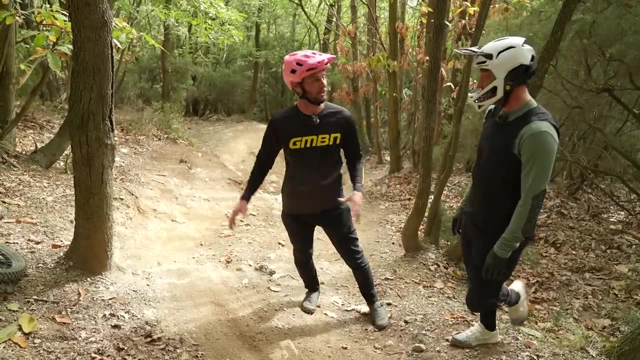 on the trail today. First up, we're going to talk about line choice, aren't we? Because you're flat out and I want to know what kind of lines you would take on a section. We've come to a very wide open bit here with multiple line choices on it. Which line would be your? 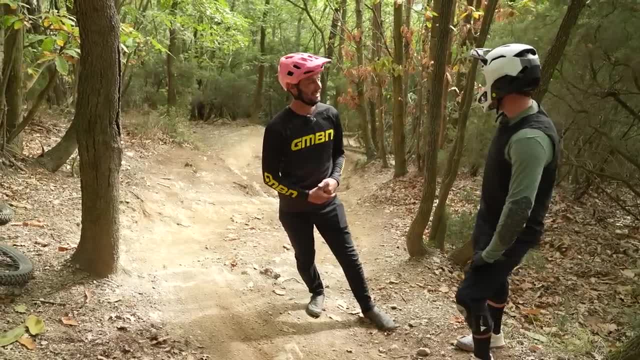 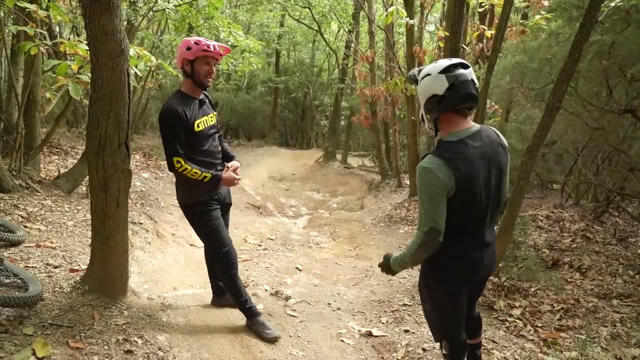 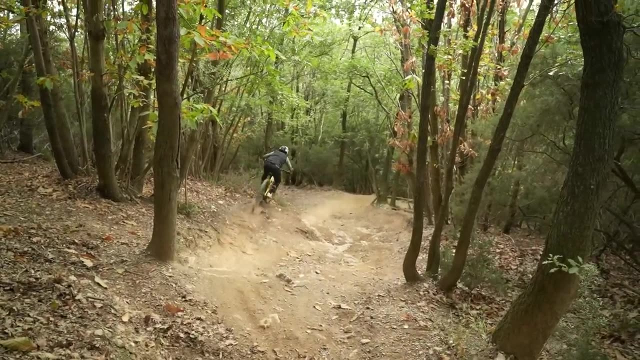 racing line and why I'm pretty sure they highlight Up on riders' left here. Yes, up on the left, so you can come in faster here, have a little brake check and then let it go on the bank. It just opens that corner. Then open the corner so you can. 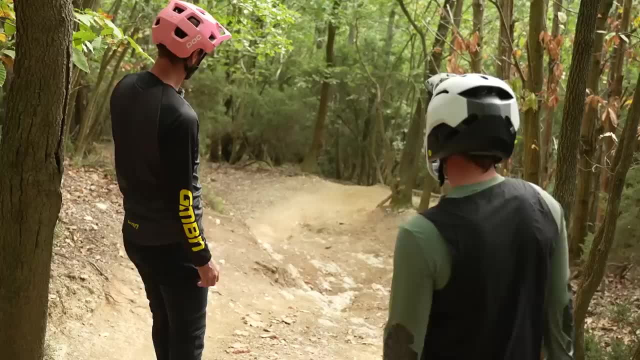 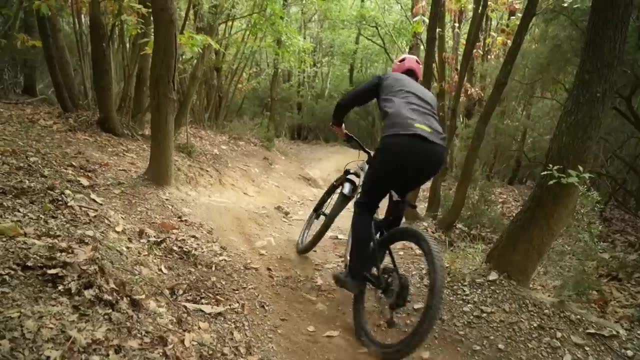 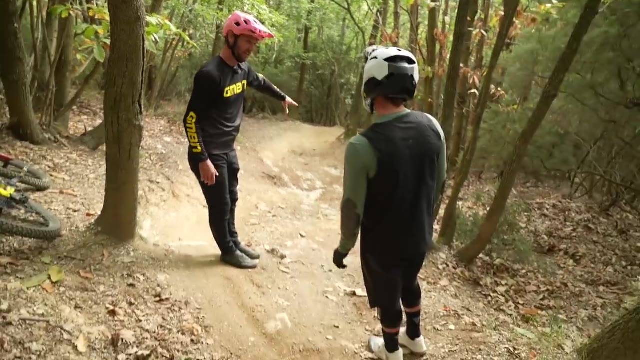 have way more exit speed. It's a quicker line all the way through like a big arc all the way through. It's only one turn. He said to do like three turns. Okay, that makes good sense, Instead of coming and slowing where you are, coming down low and then turning right here. 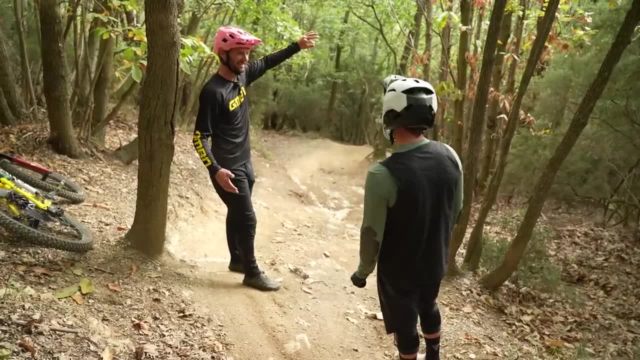 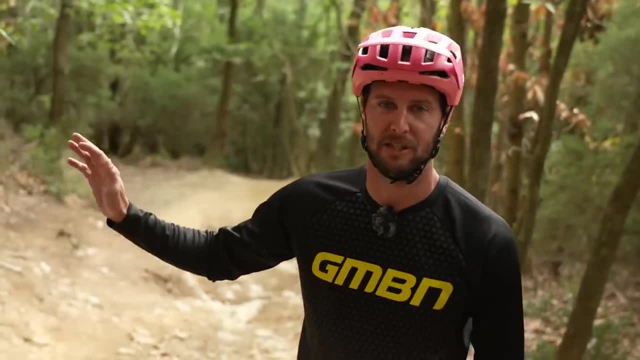 you would just go all the way around the outside, Do you fancy showing us? Yes, Come on, let's see it, dude. Let's go for it, Let's go. Okay, Loris is going to drop in. I'm expecting it's going to be pretty flat out. I'll tell you what. 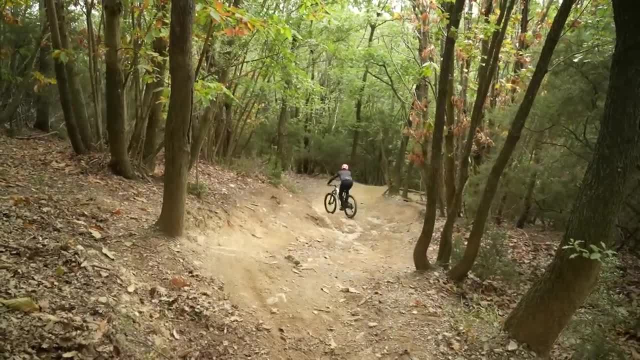 I'll go the lower line to show you the comparison as well. Okay, Loris, you're going to drop in. I'm expecting it's going to be pretty flat out. I'll go the lower line to show you the comparison as well. 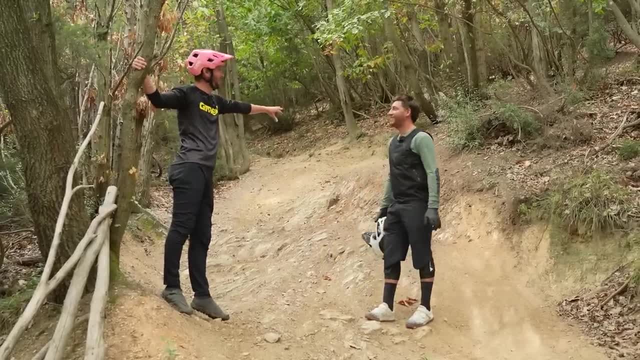 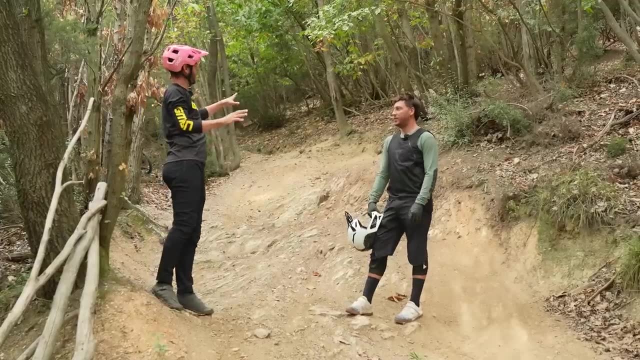 Okay, Loris, you definitely showed that this was a much faster pro line on the rider's left side there You were flying through there and really did carry a lot more speed. Is there anything else that makes you think about your line choice, or is it? 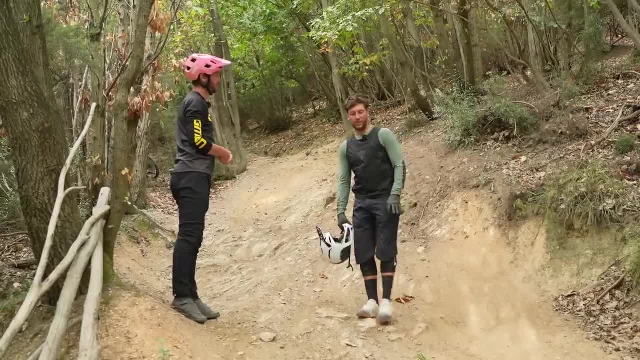 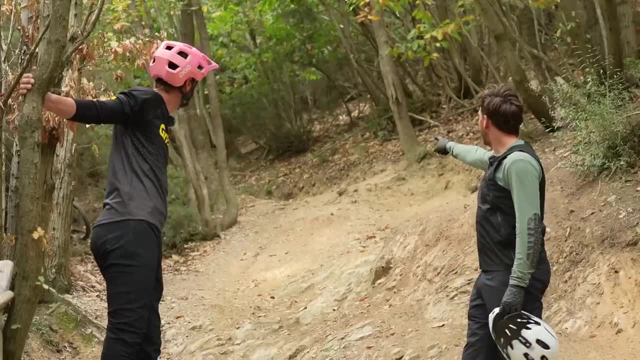 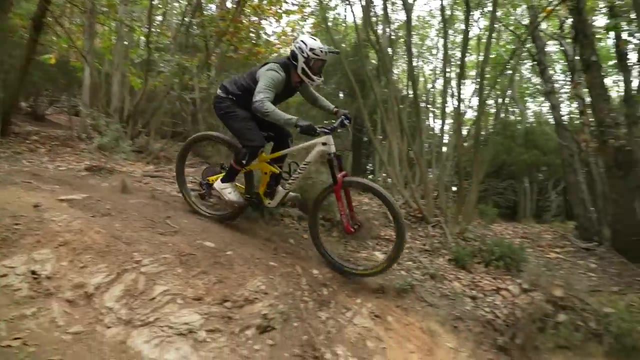 sort of just the fastest way. I think also the braking point is really it's way better than the turns because you brake just a little bit there to set up to be on the east bank and then a little brake check, Brake check here with a wheel straight, so you can carry way more speed. 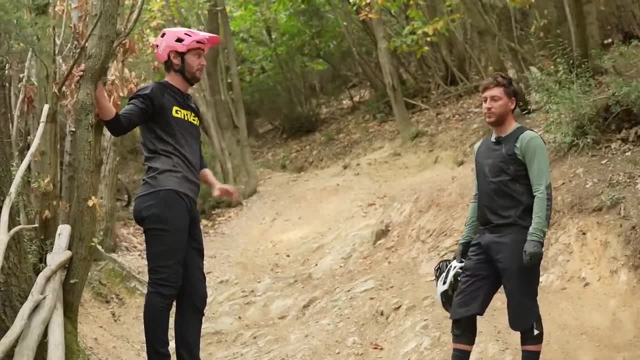 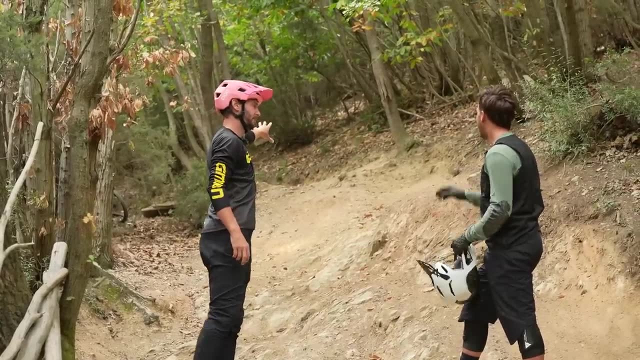 Ah, interesting. Let's dive into braking points a bit more. then You don't brake at all on this middle section here You brake before it up the top, Yes, before the top. a little bit to be perfectly set up on this one. 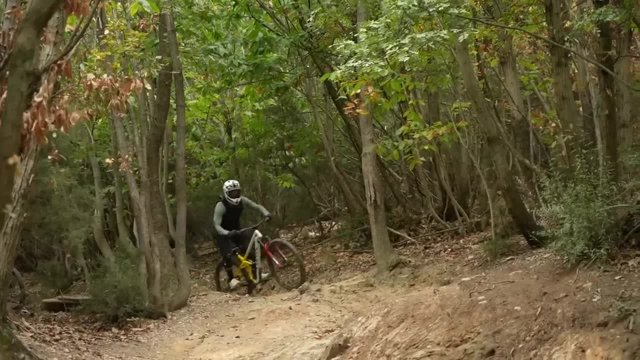 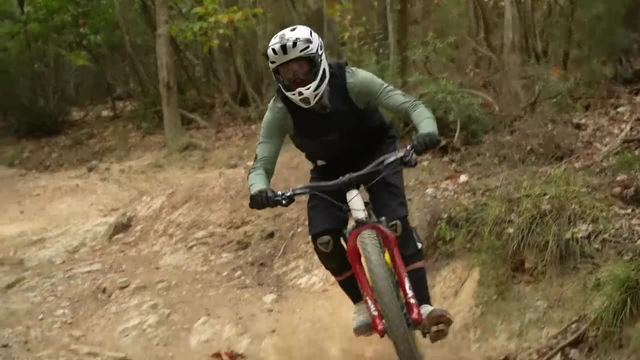 Okay, Then roll this one, Yes, and then really straight on pretty much here, and then a little brake check to have the right speed and the right positioning, and then hit the turn Just as hard as you can. Yes, As hard as it'll hold you. 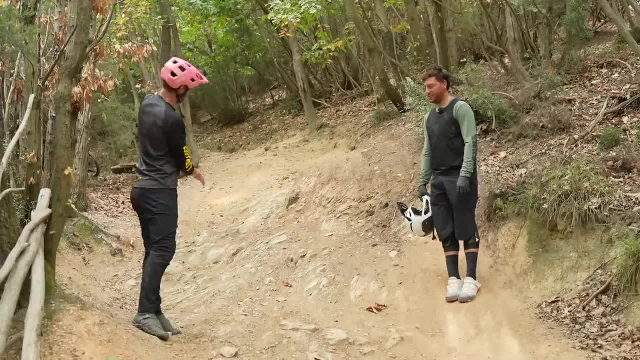 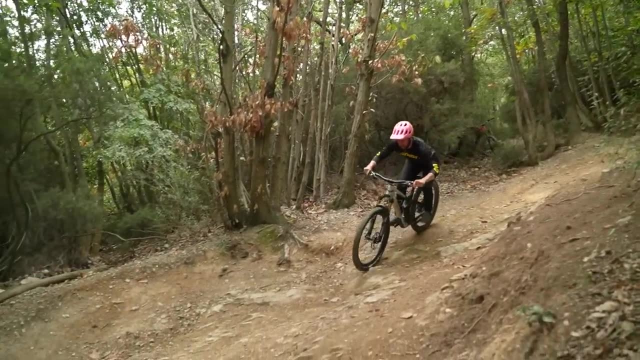 Yes, Okay Then again. so we could see, obviously from me doing this side, that because you have to come in so much tighter here that I have to brake a lot more coming into it, whereas Loris, like he was saying, he does a lot of his braking before and 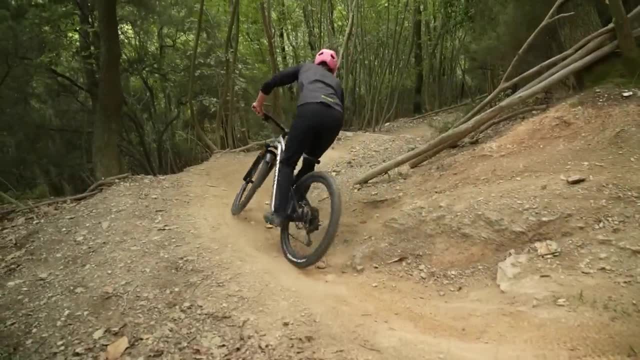 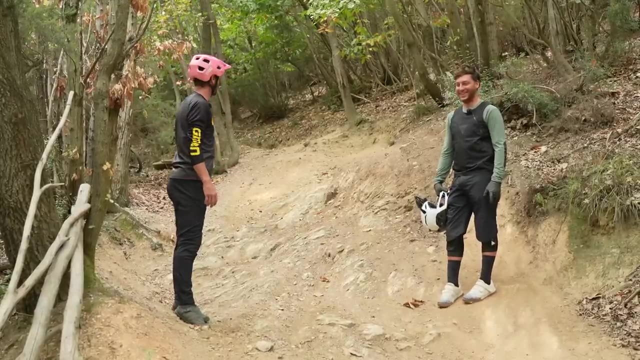 carries the speed across the top. Again, not only is it a faster line, it's faster in the sense that you brake less. Yes, also, If you're a racer, that's definitely a good thing. You don't want to be braking. 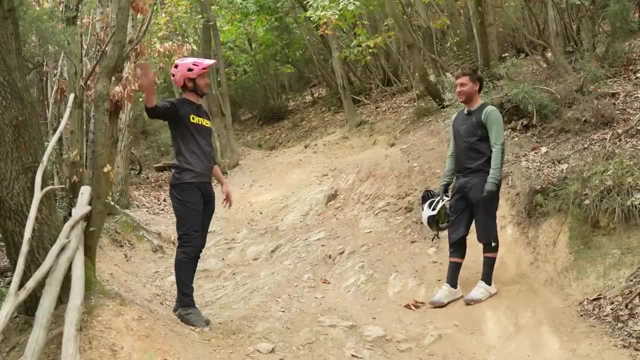 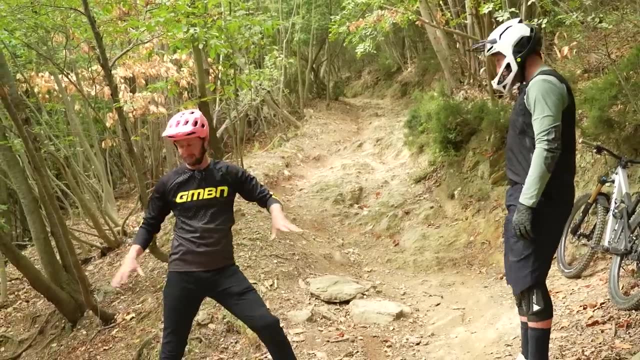 too much, All right. well, let's have a little dive further down the track and maybe look at some other sections we can try out. Okay, Nice, All right, Loris, we've got a different type of turn now because we've got a really flat out section coming in. The racing line is 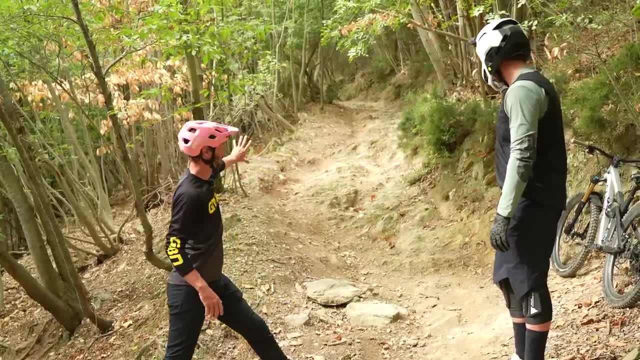 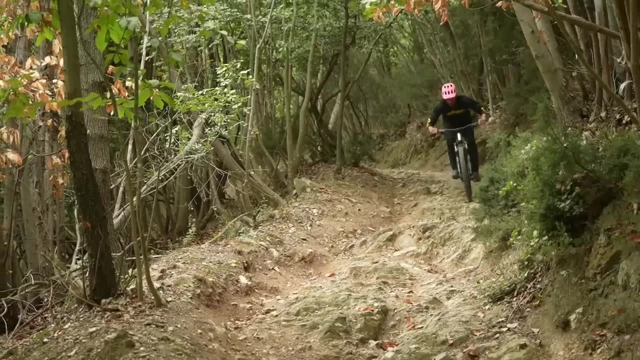 definitely to stay high If you want to avoid the rocks. you would come left or rider's right, but we're into this really tight hairpin here. then Where would you do your braking, Because I just came blasting down? Yes, I just pulled a massive skiddy drift. How would you go about it? 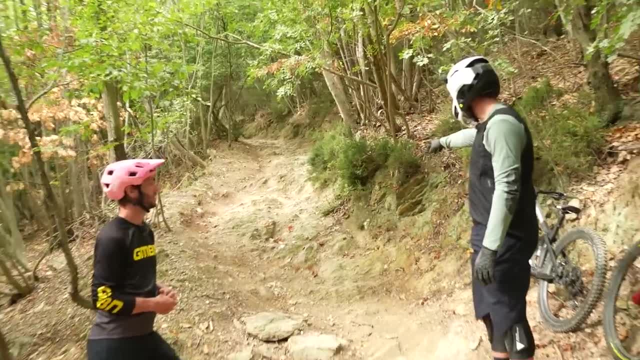 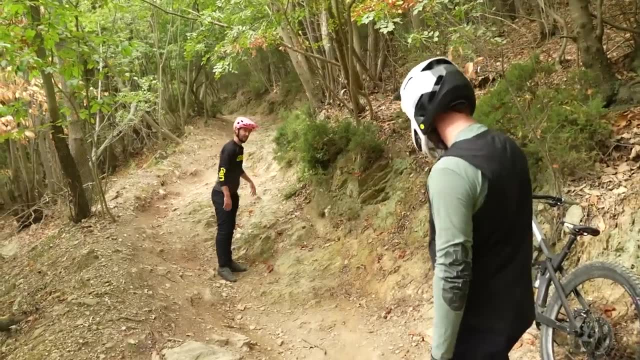 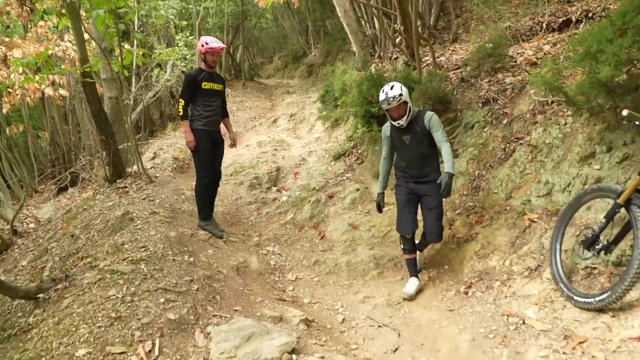 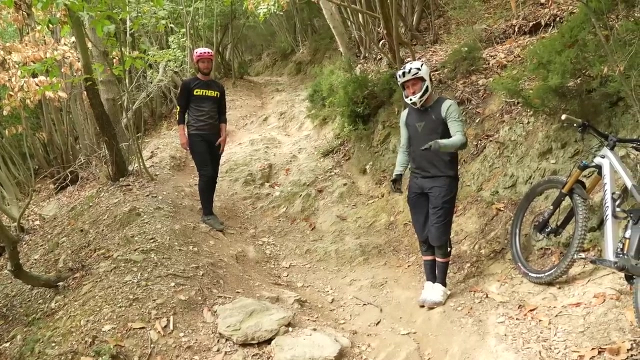 I think the perfect spot is there on the rocks, Just coming down the rock, this section here, Yes, You can have a braking point from here to maybe to here, and then let the brake go to have a maximum grip on the turn, because it's 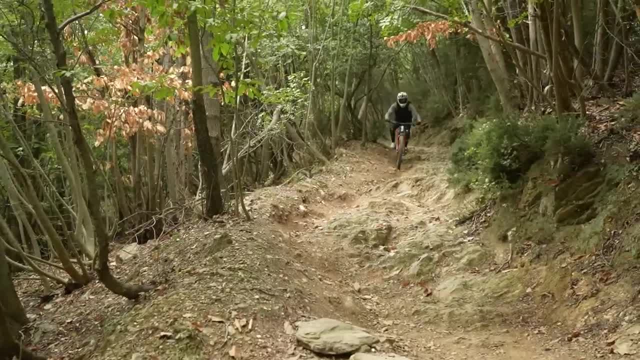 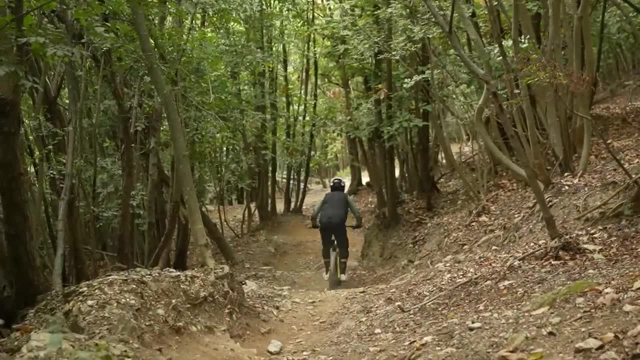 really steep and it's pretty- Oh, gravelly, Yes, Oh, I see, Rather than having, if you are hard on the brakes in the turn is when you might lose traction. is what you're saying? Yes, exactly, When you change the speed of the wheels, you always lose grip. 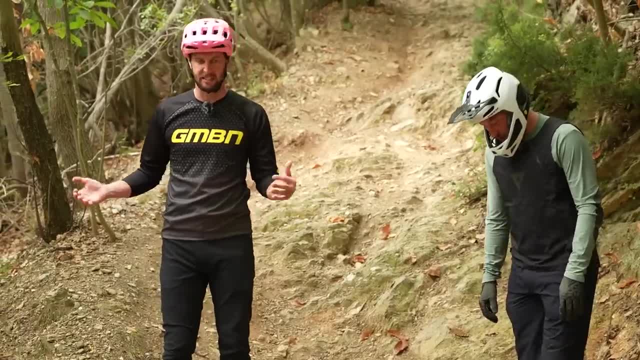 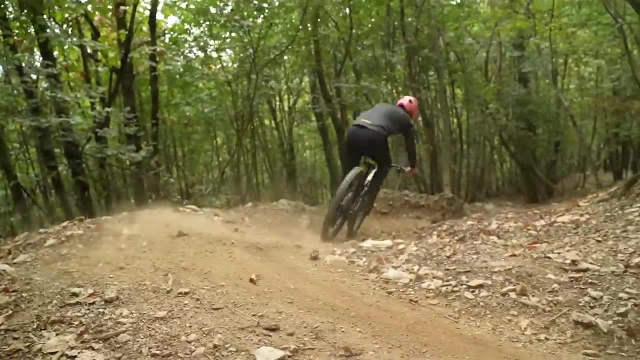 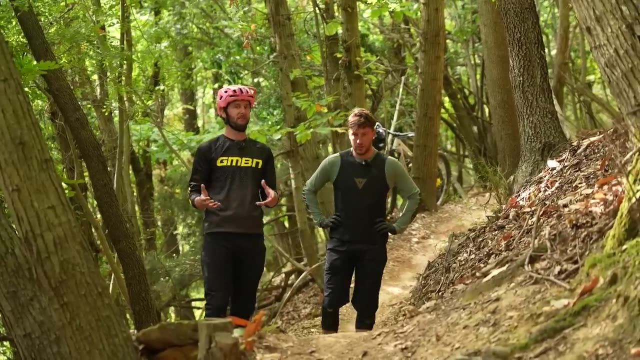 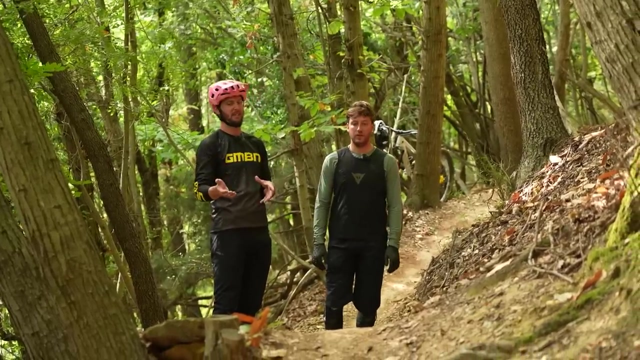 Okay. Well, let's see you blast through it and see how it's done. All right Now. pre-hopping is essentially bunny hopping over something to go faster, I would say. Would you agree? Yes, It is. The jumps and rocks and obstacles are great examples of this. We've got a jump. 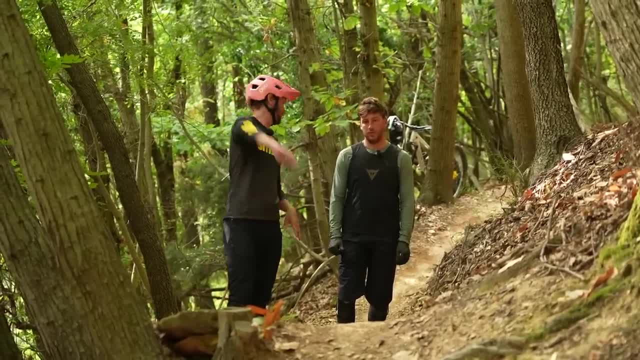 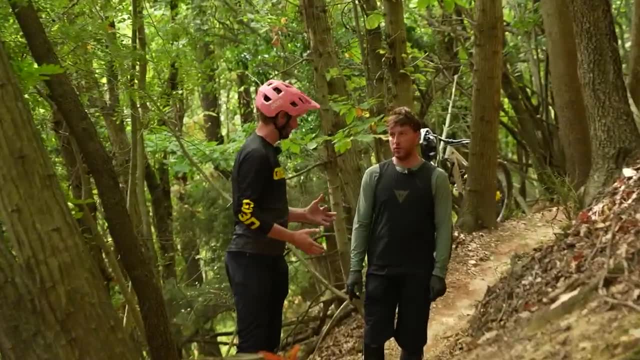 here, which normally you would blast it down the trail and just send it off the jump. Yes, The fastest thing to do, which Loris is going to show us, is to pre-hop it To run us through, Loris, what you're going to do. 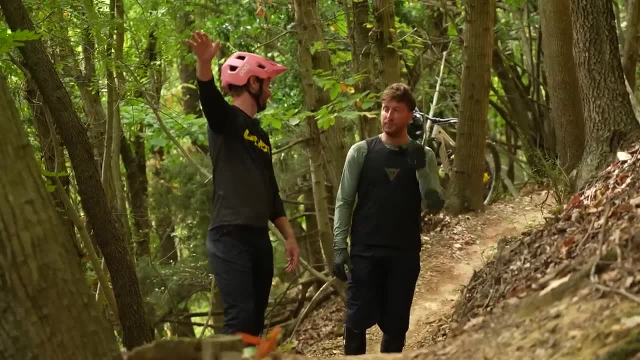 from here onwards, because I'm just going to send it one. Yes, I'm going to go send it on. Yes, Go ahead and jump almost. Yes, You're going to go. Yes, Yes, You're going to go. Yes, You're going to juxtapose that. 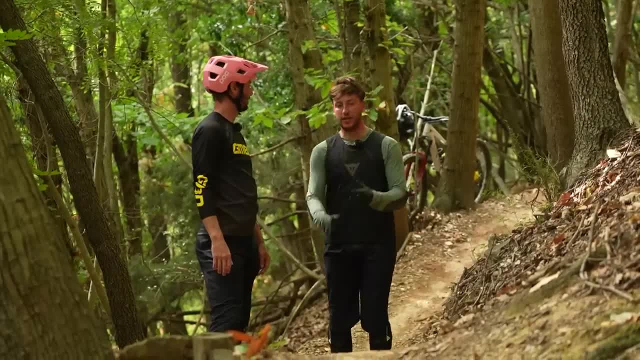 Yes, All right, then you're going to jump. Yes, Yes, that's like a pretty fast section. If you just hit the takeoff, you're going to- Yes, go miles. Yes, and you want to hit that-. 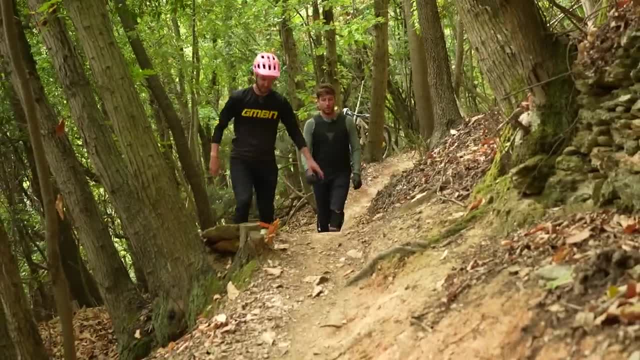 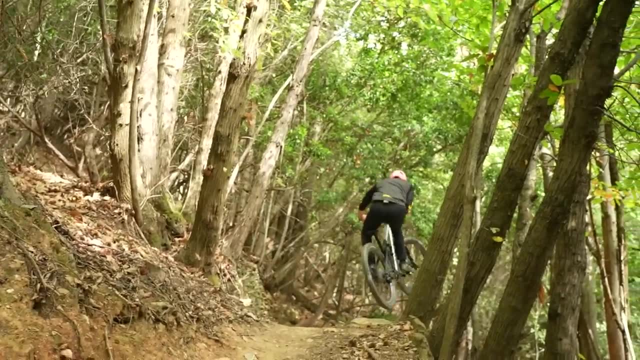 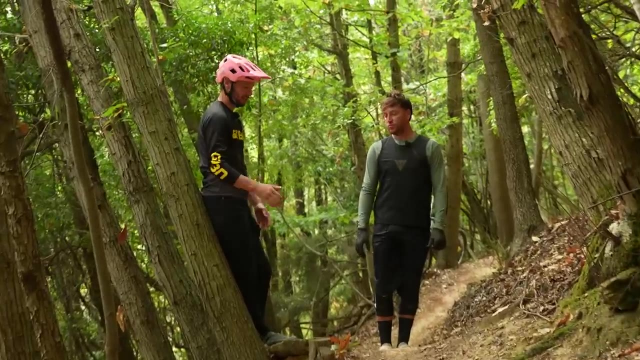 On the backside. Yes, You're aiming to, actually, because I'm going to take off here and I'm going to land down here somewhere. Yes, which is pretty flat. Yes, I want to backside this one. Yes, can I have a pump and increase my speed? You're not looking to just not lose speed. 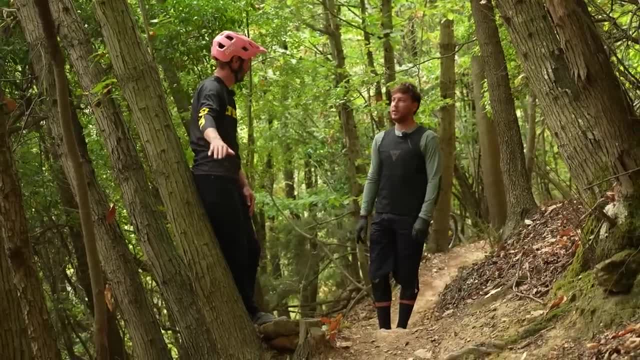 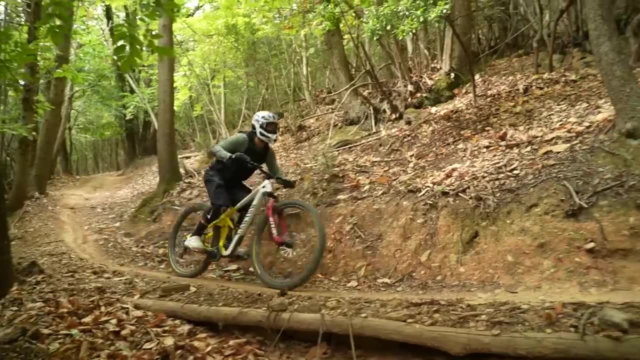 from jumping in the air. You're actually looking to go faster. Yes, I try to be faster, Yes, and I guess if you do this, maybe once, two, three times on a track or a race run, all those little bits of time will add up. 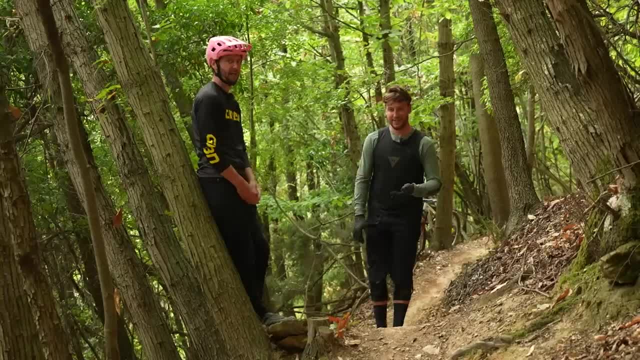 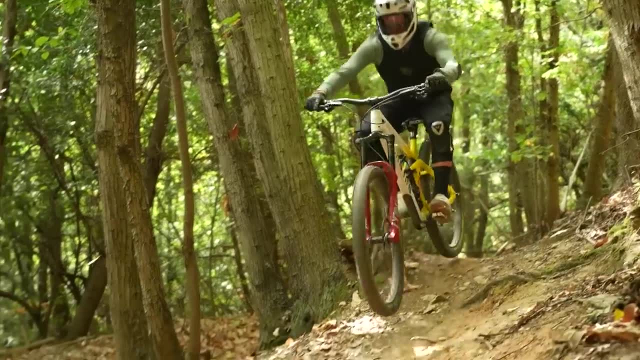 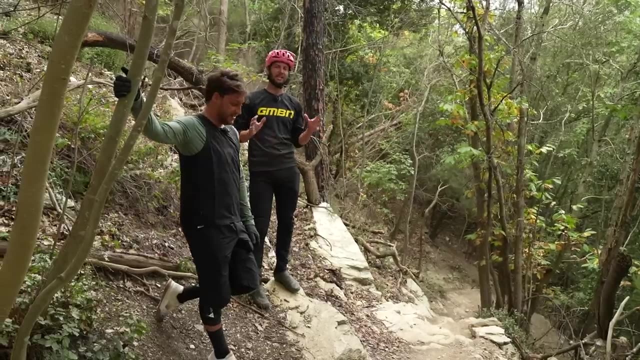 Yes, that's right. Okay, good top tip there. Let's see how it looks in real life, though. Right, I've brought us to the next section because we're going to talk all things unweighting Now. when you see a proper flat out rider go through a rough section. 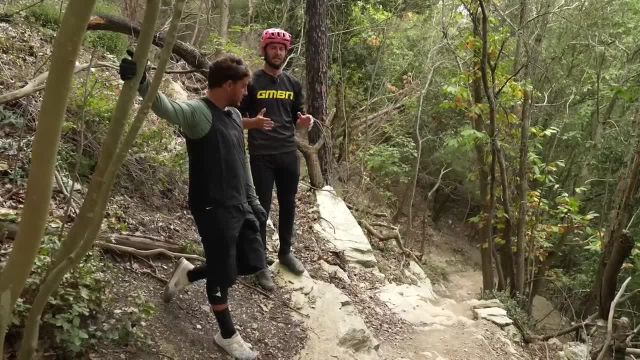 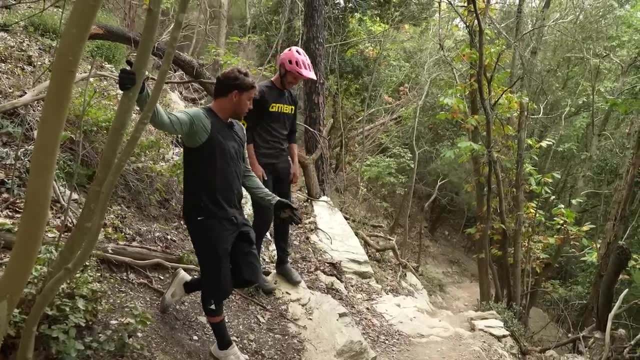 you wonder how they make it look so smooth and how they're not destroying their bikes. What they're doing is unweighting the bike, and Loris is going to tell us about that now. Yes, we're going to use that pressure here, This bit in the middle. 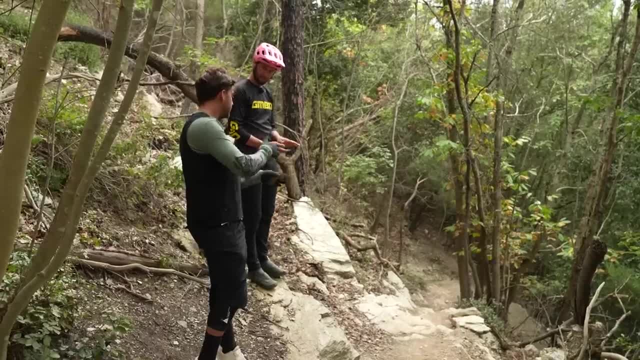 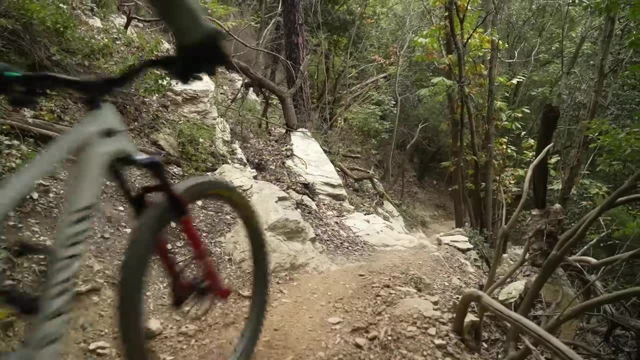 Yes, The bike is going to compress and then when you release, when we are at the top of the road, the suspension is going to release the pressure. Yes, Like its longest point. Yes, and we're going to extend the body and we try to be light on those rocks and-. 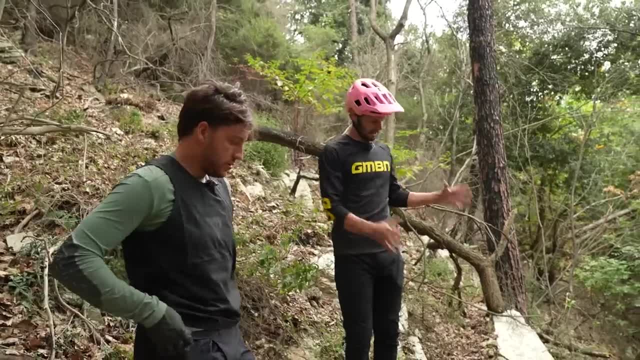 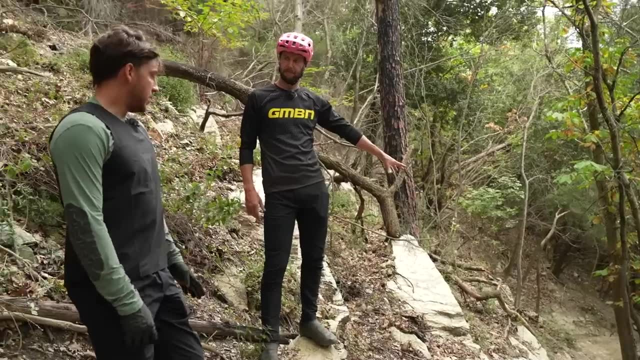 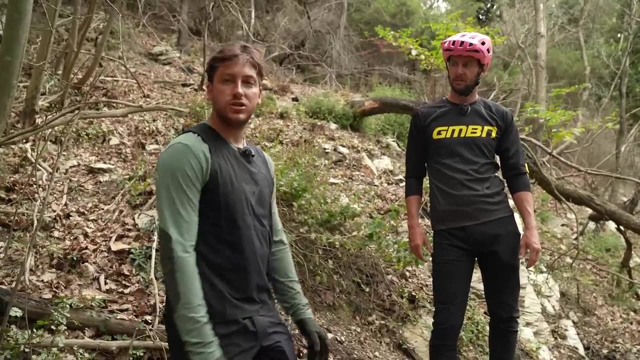 And just float through it. Yes, Float, Tell me, Loris, rather than just hammering through. why would you try and unweight the bike on something like this to get through it? Smoother, it's faster, It's also safer and less punctures Also, you can save more energy. 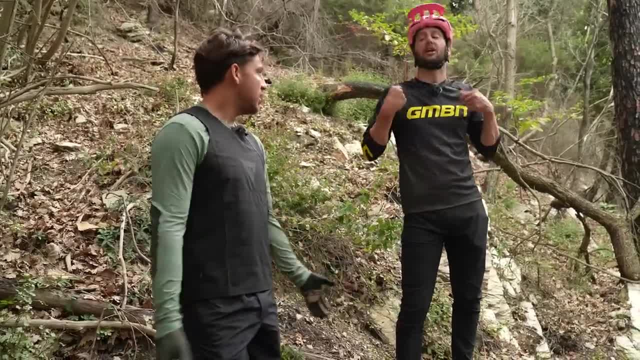 Yes, Because you're not needing all the holes and- Oh, so you're not just constantly like that all the time. Yes, You can have more energy just near the bottom. That sounds good to me. Okay, let's drop him. 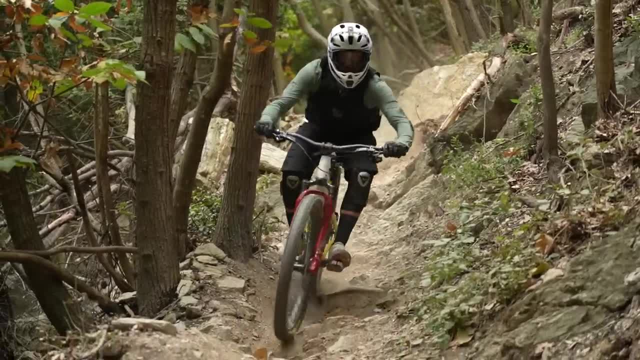 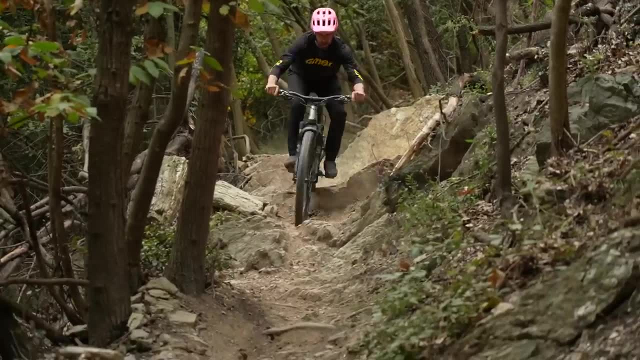 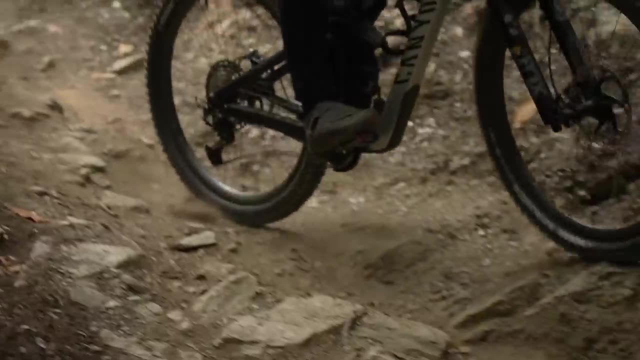 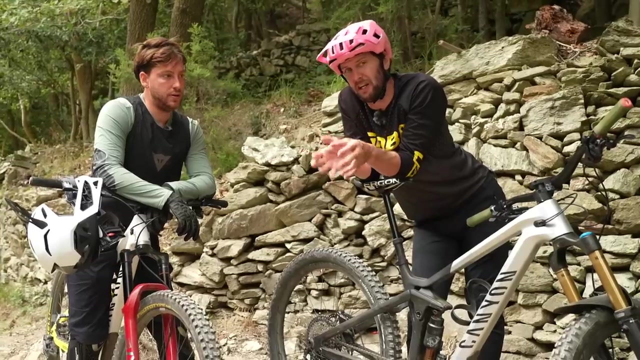 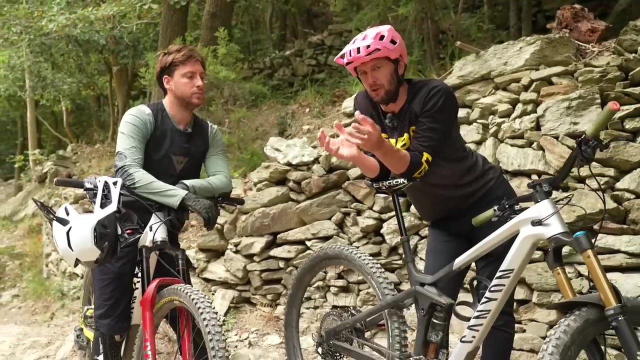 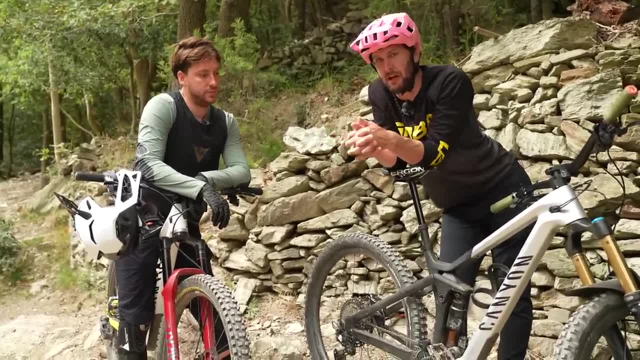 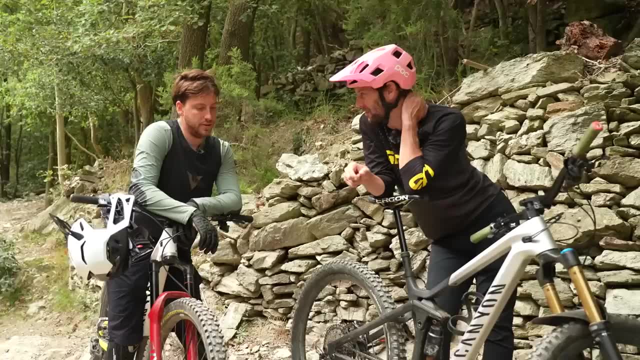 is pretty tricky. It's a tough place to get yourself into to not buckle. Let's hear Loris: how do you get into the mindset to focus for that one run and go as fast as you can? I start from the first day of practice to 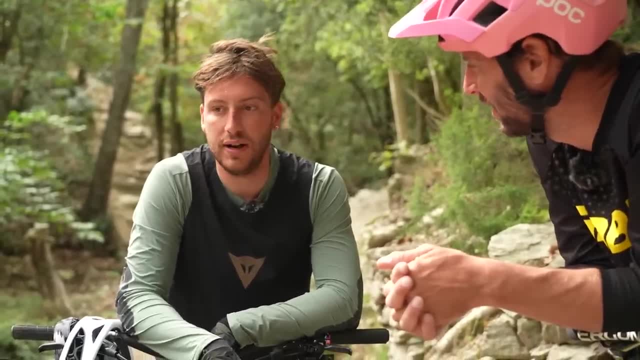 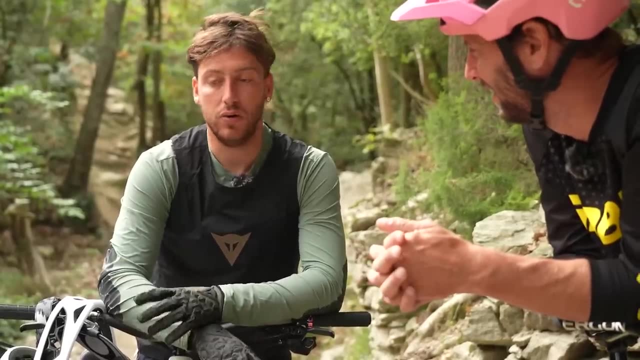 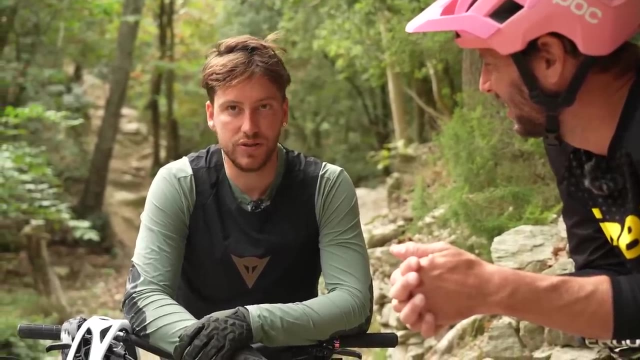 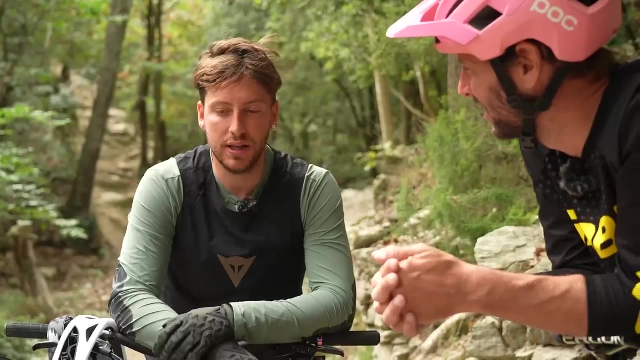 try to enjoy the track and have fun. When you have fun, you're way more chill than when you be like, oh I'm struggling. Try to be really relaxed. Then, before race run, I use a bit of music and I like a joke with my mechanic. We do some exercise together and just enjoying. 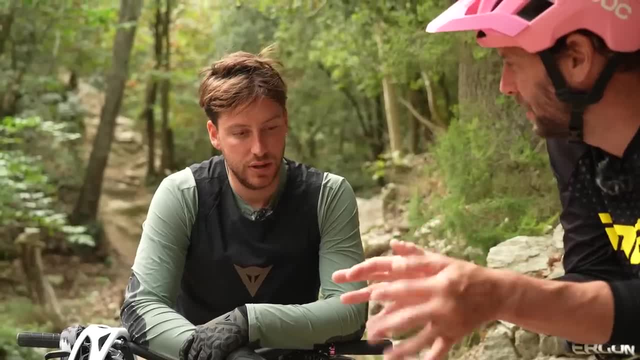 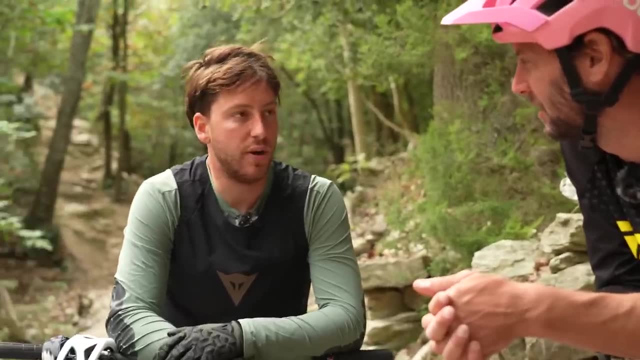 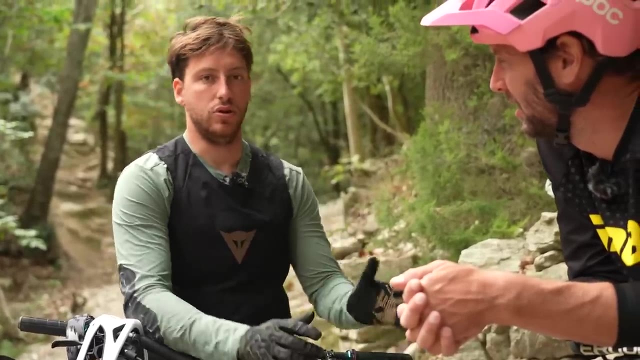 Yes, Do you have like a set routine that you always do, or is it changed from race to race? No, it's pretty much the same. I go at the top one hour before the final and then 40 minutes before I start to warm up. Then I take 10 minutes to visualize the track.